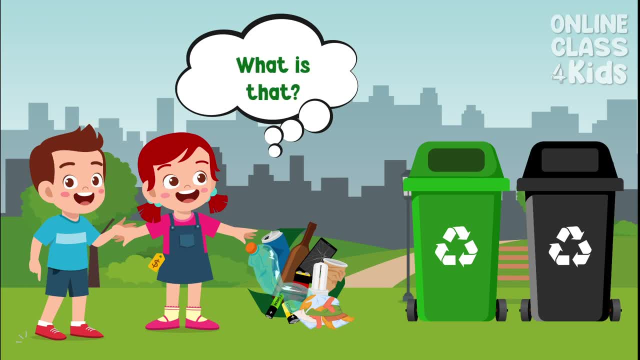 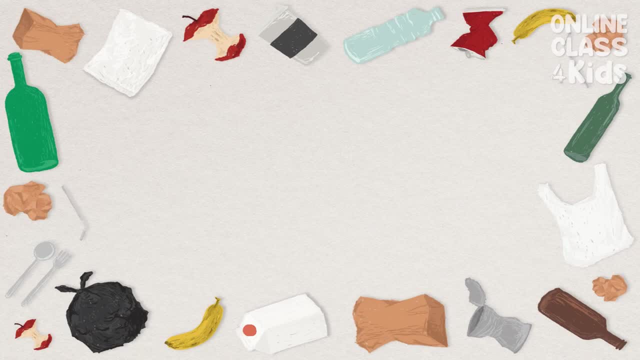 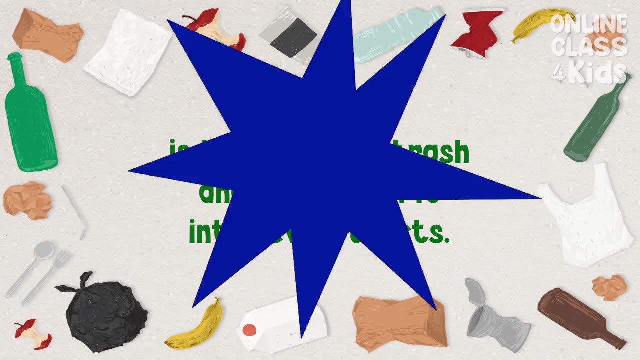 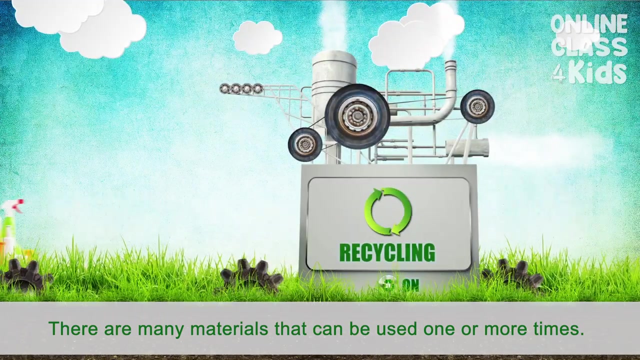 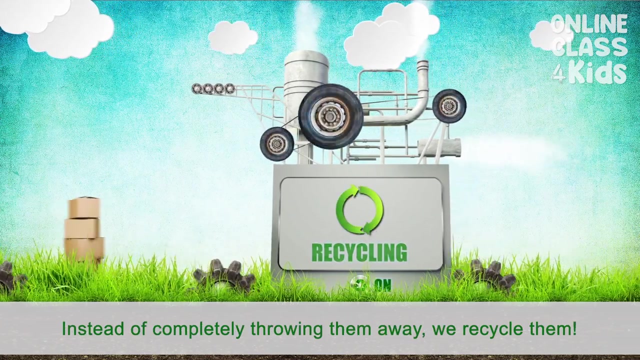 Recycling bin. What is that? Let me tell you more about recycling. Recycling is how we take the trash and transform it into new products. There are many materials that can be used one or more times. Instead of completely throwing them away, we recycle them. 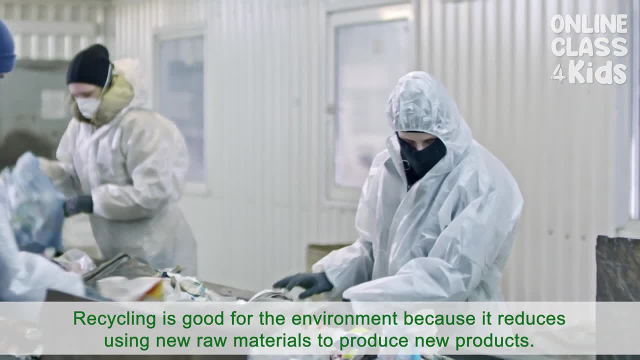 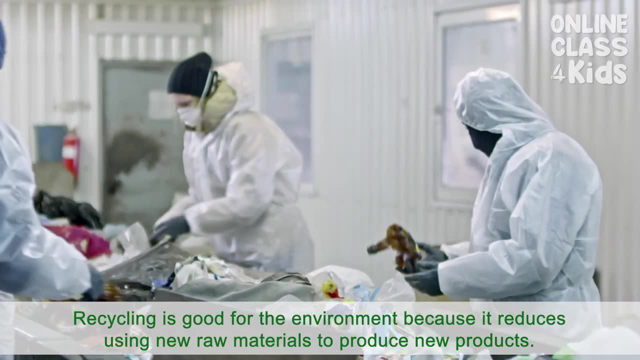 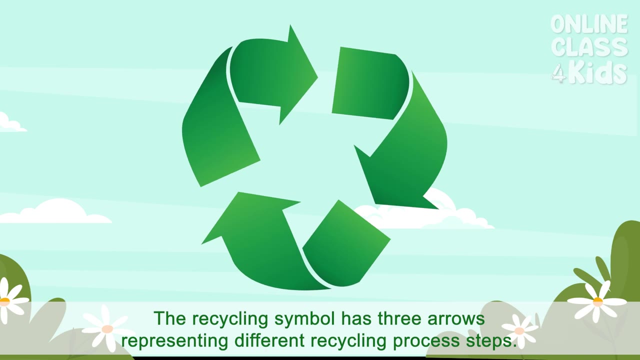 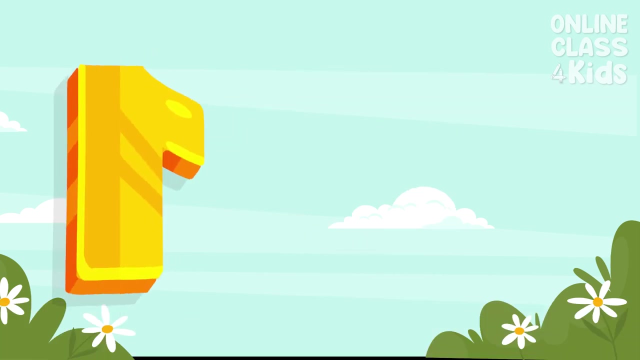 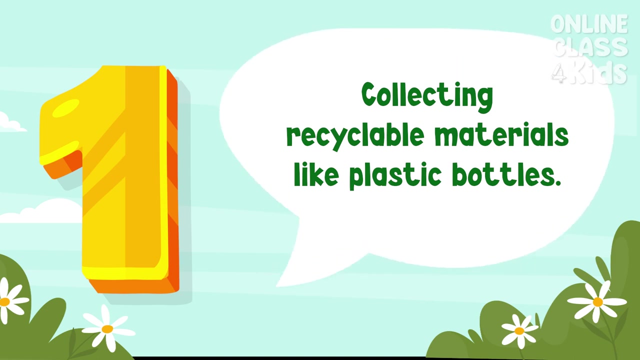 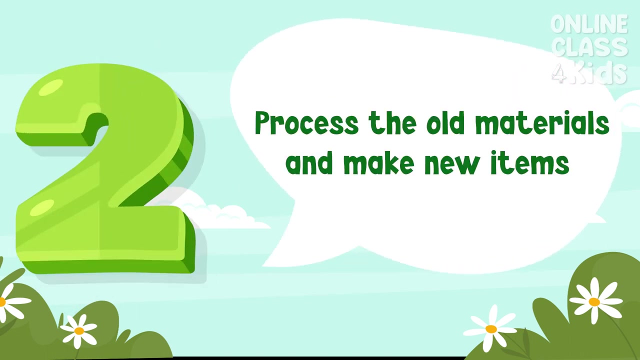 Recycling is good for the environment Because it reduces using new raw materials to produce new products. A recycling symbol has three arrows representing different recycling process steps. The first arrow means collecting recyclable materials like plastic bottles. The second step is to process the old materials and make new items. 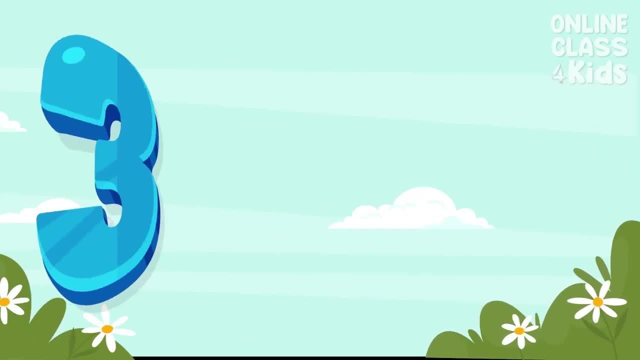 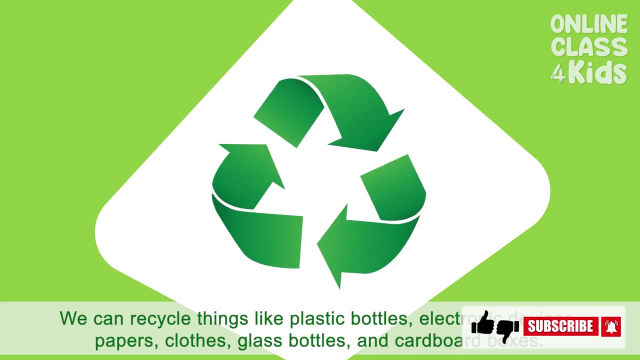 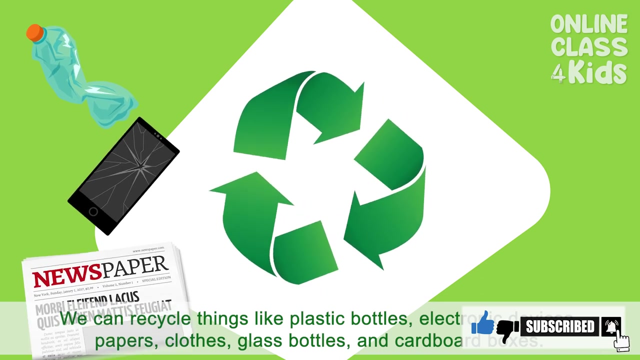 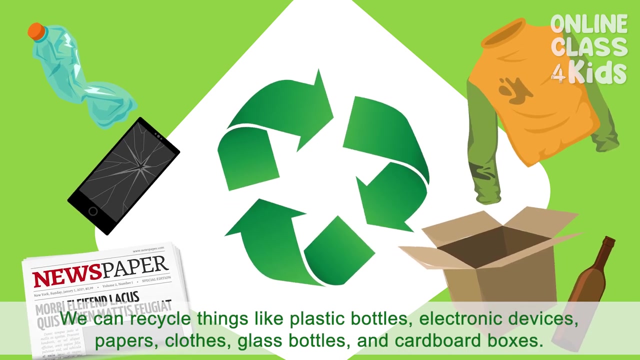 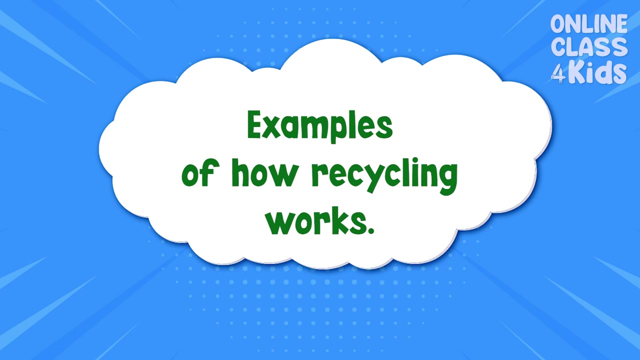 And finally, the third step is buying items made from recycled materials. We can recycle things like plastic bottles, electronic devices, papers, clothes, glass bottles and cardboard boxes. Here are some examples of how recycling works. One plastic soda bottle can be recycled into planters. 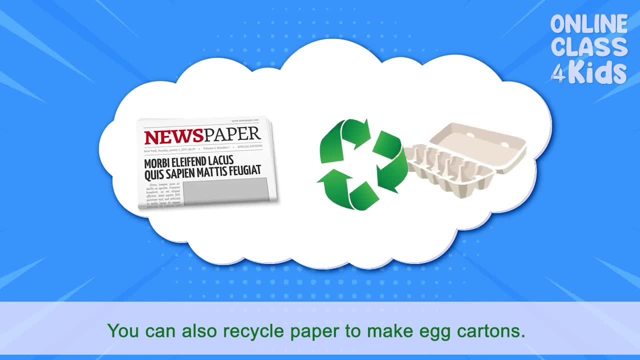 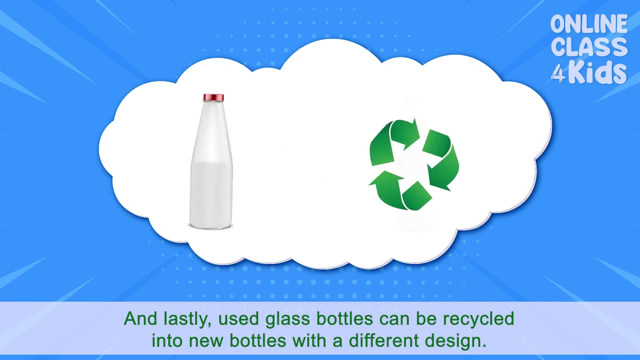 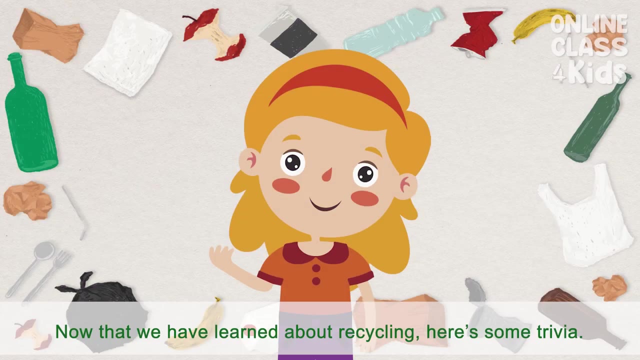 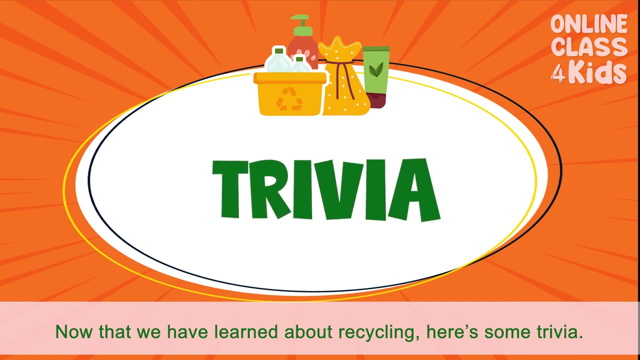 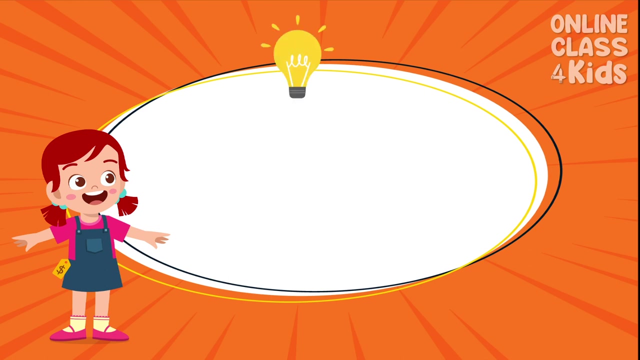 You can also recycle paper to make egg cartons. And, lastly, used glass bottles can be recycled into new bottles With a different design. Now, that's what we have learned about recycling. Now, here is a trivia: The energy saved from recycling a glass bottle can light a light bulb for as long as 4 hours. 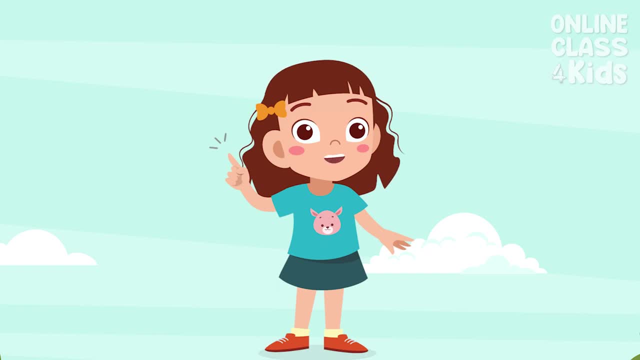 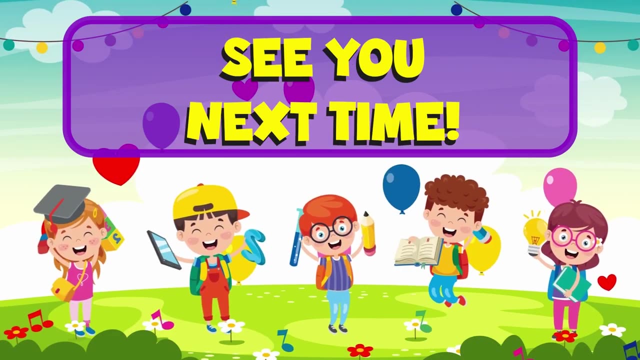 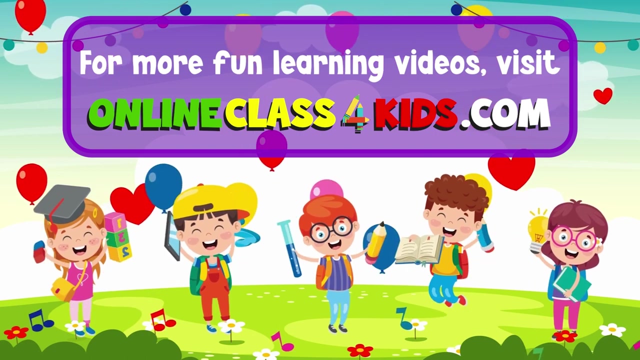 I hope you had a wonderful time learning about recycling. See you next time for another fun-filled learning, only here at Online Class for Kids. Visit OnlineClassForKidscom for more fun learning videos and don't forget to subscribe to our channel.